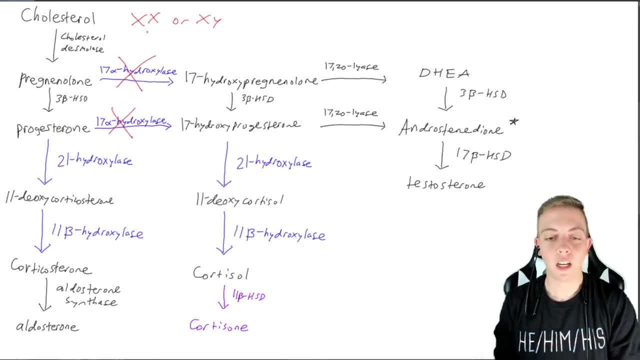 going to talk about the differences just yet, because it'll come in the presentation and the pathway is going to be the same for both. But we have cholesterol. Cholesterol is going to enter and be converted by cholesterol desmolase to pregnenolone, same as we would always have. 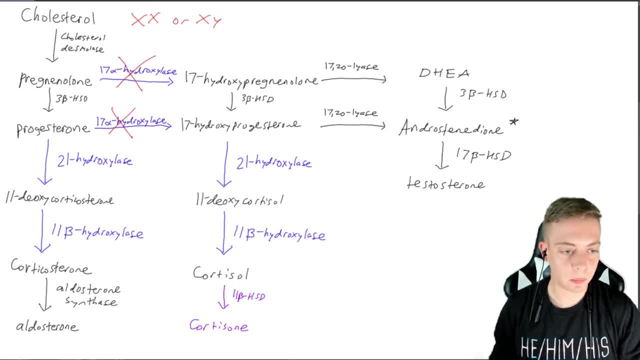 I'm going to change my color really quick, just so it looks a bit different. So we have cholesterol. we have cholesterol desmolase, so we are going to make pregnenolone. We have 3-beta-HSD that is functional. So we are going to produce progesterone And the rest of this pathway is okay. We have all of these, So we can go through all the way to aldosterone. So we, unlike the last two pathways where we had no aldosterone, we do have aldosterone, But let's say we needed to make some cortisol. So let's say we have some inflammation that we want to get rid of, or we're in a time of stress and we need some cortisol. We can't go this way because we don't have 17-alpha-hydroxylase, which is our common enzyme to go from pregnenolone to 17-hydroxypregnenolone and also from progesterone. 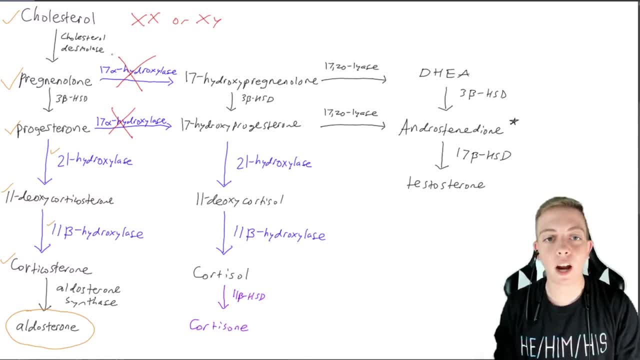 to 17-hydroxyprogesterone. So we can't at all go to this cortisol pathway. So we can't do this, Can't make this either. We can't make 11-deoxycortisol, We can't make cortisol and we. 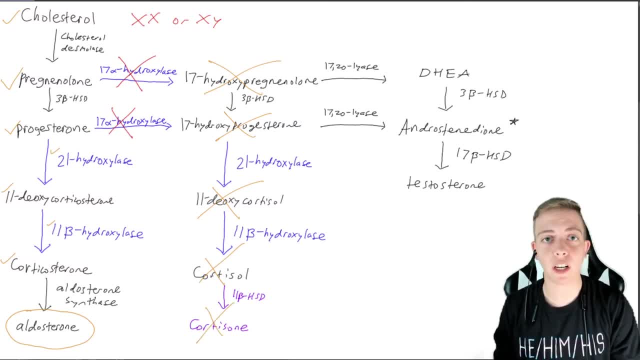 can't make 17-hydroxycortisone, So we're going to have some issues with inflammation and with times of stress and blood sugar. But can we use our 17-20 lyase? No, because we couldn't take this. 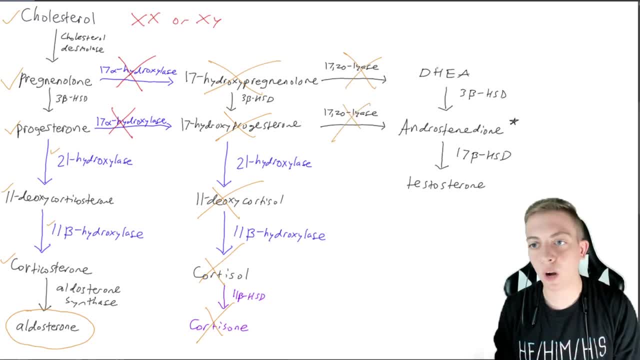 initial step to even get there. So all of this is also irrelevant. So we can't make DHEA in the adrenal gland, We can't make androstenedione and we can't make testosterone here. And let me give you a little bit of a disclaimer, because this, this is something that happens in the 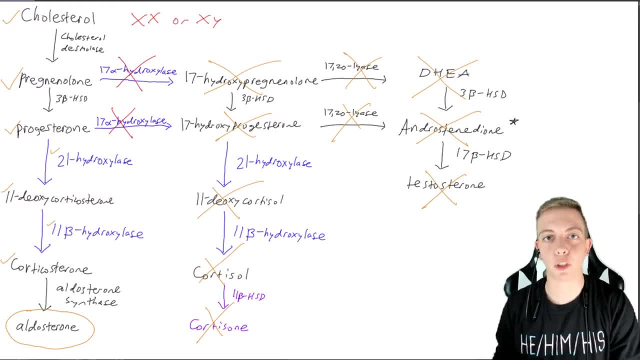 adrenal gland, but we do have alternate pathways elsewhere to make androgens, especially in the testes. We have a different process there, And then we also make some testosterone in the ovaries as well, And we're going to cover all of that. So you're not going to be entirely without androgens. 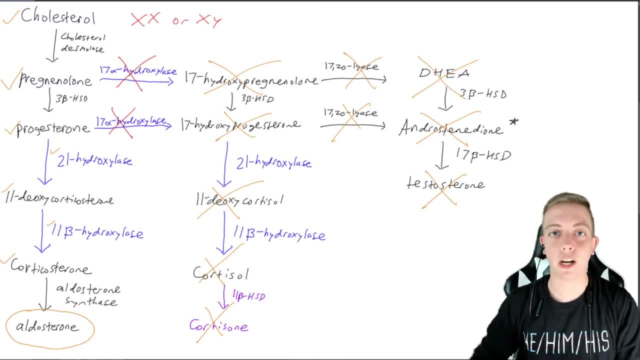 but you're going to have a significantly decreased level of androgens compared to somebody else without this deficiency. So, as you can see, we have no cortisol and we have no androgens from this pathway, but as all of this is going to back up because we can't go forward, So now we have. 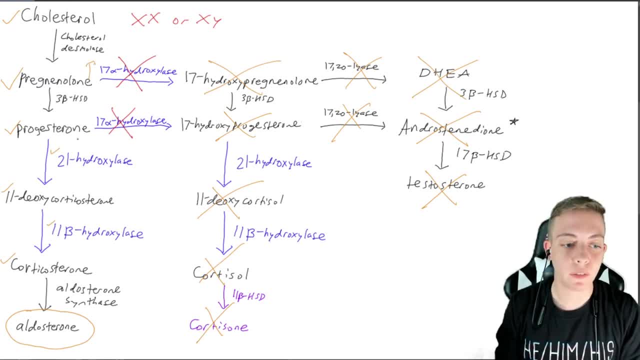 to go backwards. So now we're going to have increased pregnenolone, We're going to have increased progesterone, We're going to have increased 11-deoxycorticosterone, increased corticosterone and increased aldosterone. So we're going to have a lot of aldosterone And, if you 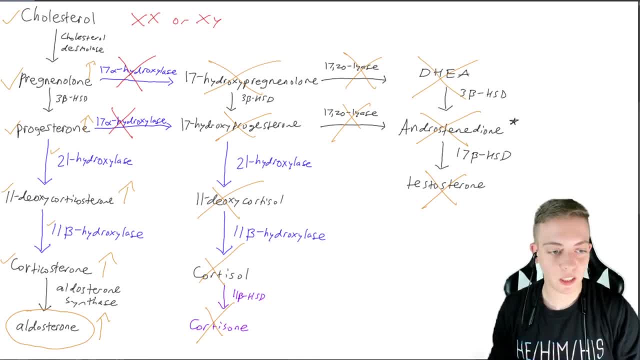 remember what aldosterone does, you will be able to figure out how this presents. So let's write this all out, Our presentation. Let's say we have an XY fetus that has an SRY, So we're going to assume that this is XY plus SRY. They're going to have ambiguous genitalia and they're also going 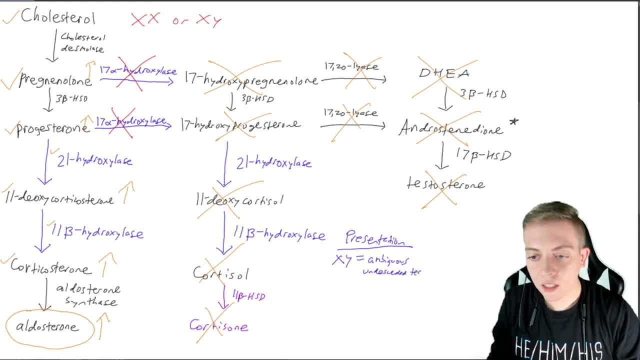 to have ambiguous genitalia Because testicular descent is related to testosterone and related to DHT. that is what stimulates the testes to descend. So we're going to have testes inside of the abdominal cavity and we're going to have ambiguous genitalia. It's going to appear more feminine than 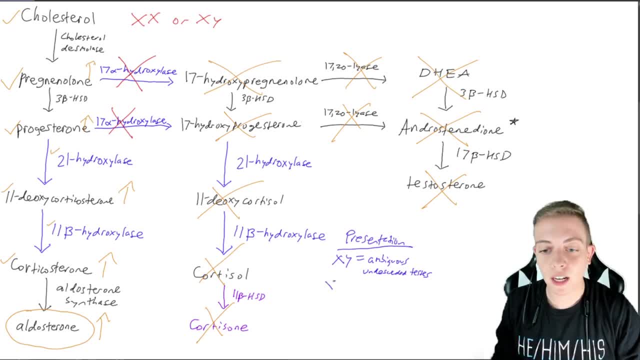 what you would typically see with an XY fetus And then an X fetus. So we're assuming somebody without SRY. Okay, They're going to present, typically how females would present. They're going to have external female genitalia and internal female genitalia, but they're going to lack secondary. 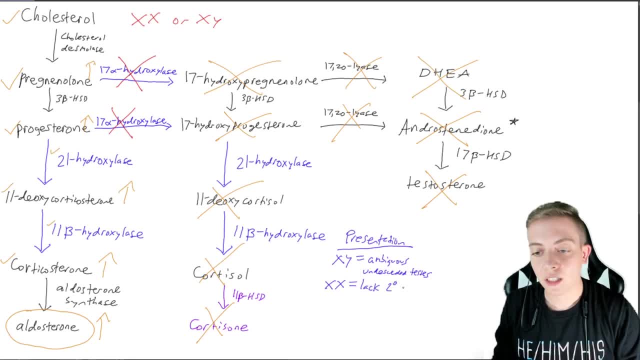 development. So this means when they hit puberty we do see some androgens being produced and those do actually play a role in female puberty. So not having this testosterone or androstenedione is going to make an XX person develop less so than somebody who has an appropriate amount of androgens. So we're 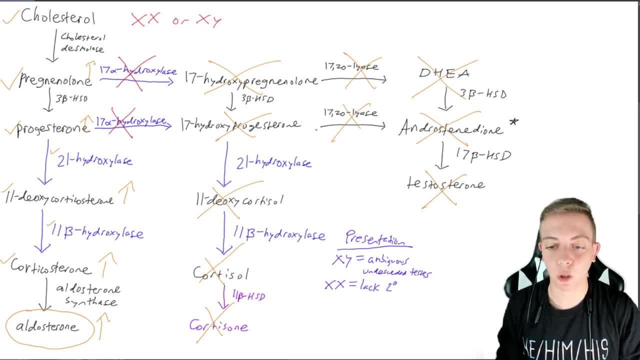 going to have less sexual development in someone who is XX. And then just adding our other factors here, Wow, I cannot Right. Our aldosterone level is going to be high, very high, because that's where all of our cortisol is being shunted to. We're going to have low cortisol And we're going to have low androgens.